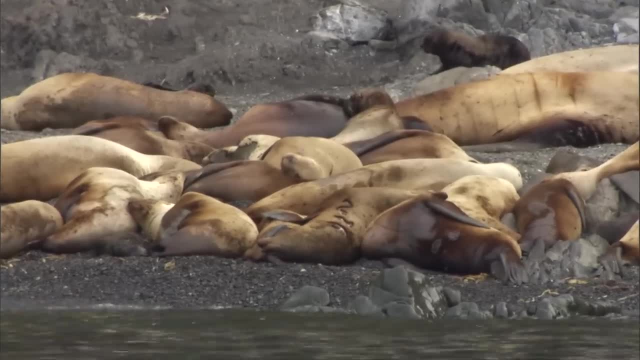 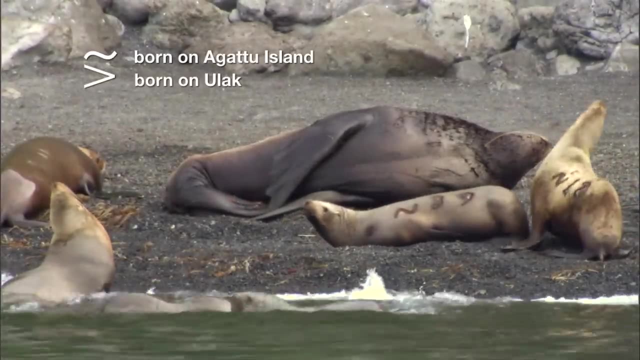 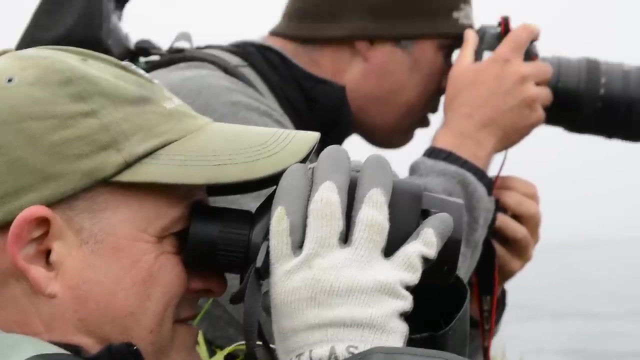 for previously marked animals and, depending on the conditions and site survey, from land or from a small boat. Different prefixes correspond to where these animals were born and, year after year, valuable data starts to illustrate trends like what percentage of pups survived to adulthood. 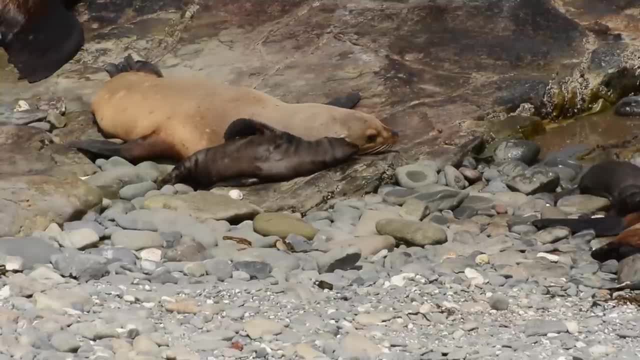 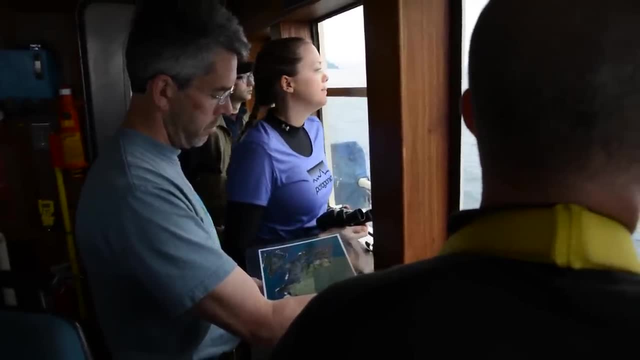 And how old a female is when it has its first pup. But covering dozens of sites over hundreds of miles in two weeks leaves lots of gaps in the data. A few years ago, we started putting remote cameras on some of our stellar sea lion haulouts. 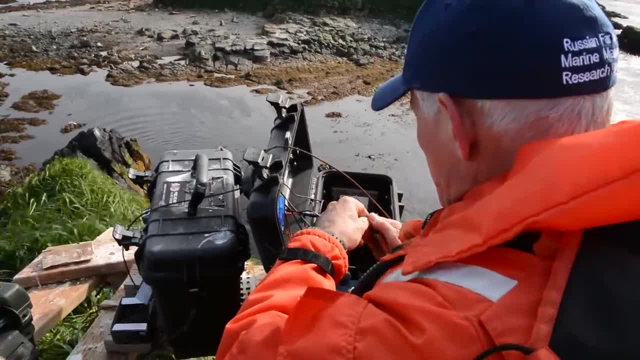 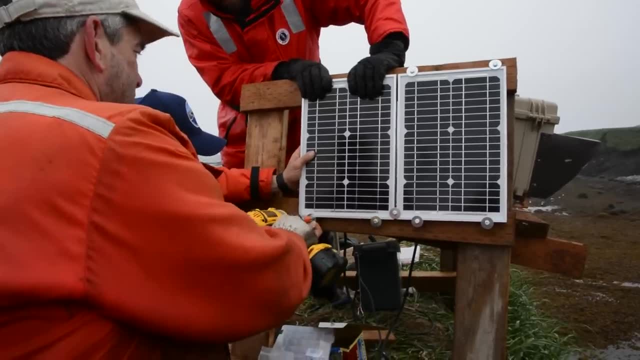 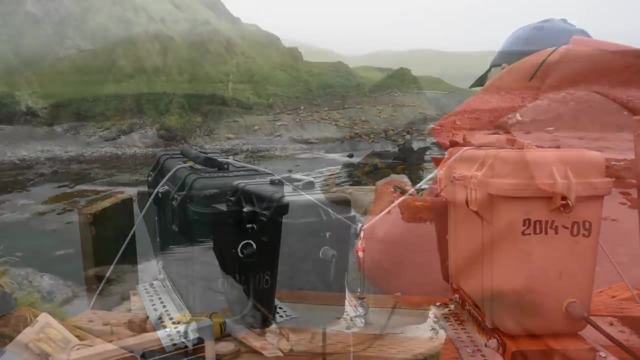 and rookeries. The cameras are put into watertight housings. We sometimes have to build temporary structures to hold the cameras, And they're set to take a photograph every 10 minutes or 15 minutes, whatever interval we need During daylight hours, in perpetuity. So those images, hopefully, will provide us a couple 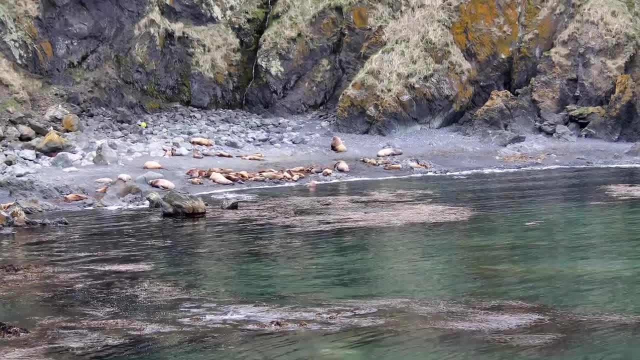 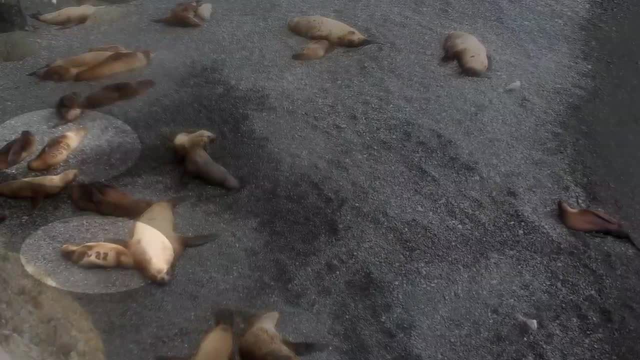 of things. One is that they can give us counts, daily counts, of some of these areas. We're also using the cameras to look for marked sea lions, And some of these animals roam quite a distance, and so we're able to identify those animals, including some from the Commander. 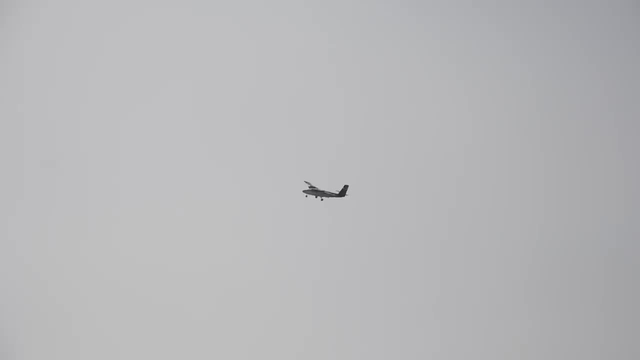 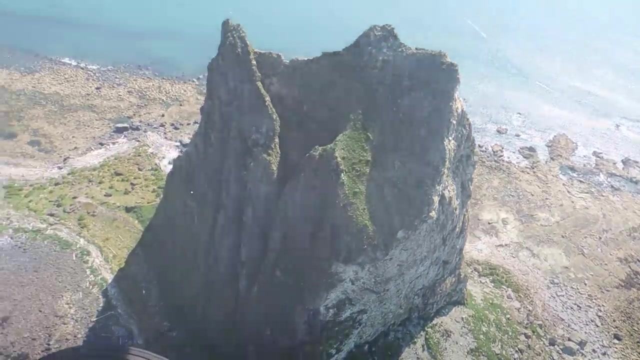 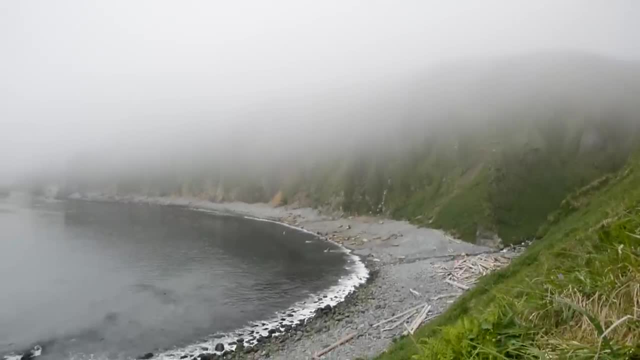 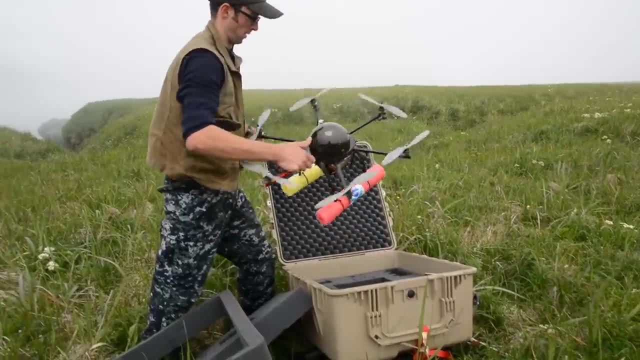 But most years this data set is incomplete, Because summertime in the Aleutians usually means fog. So one of the new pieces of equipment that we have this year is an unmanned aircraft, a hexacopter, which allows us to be ready to deploy when the fog or the ceiling lifts. 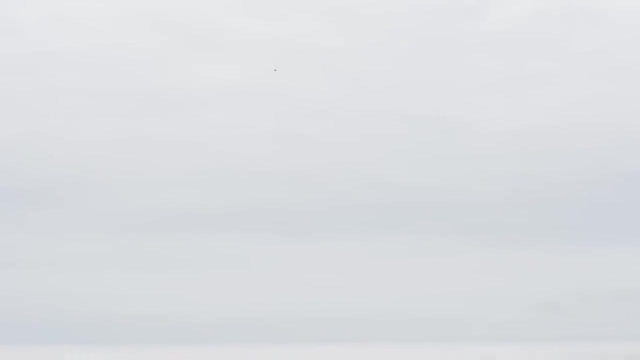 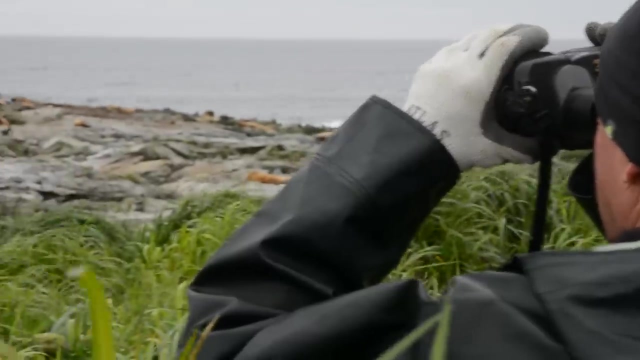 something that a Twin Otter would never be able to do. It also allows us to look at sites that, even with researchers in the field of binoculars, we can't see. Some of these sites are very flat low islands and there's just no elevation for a person, So we're able to. 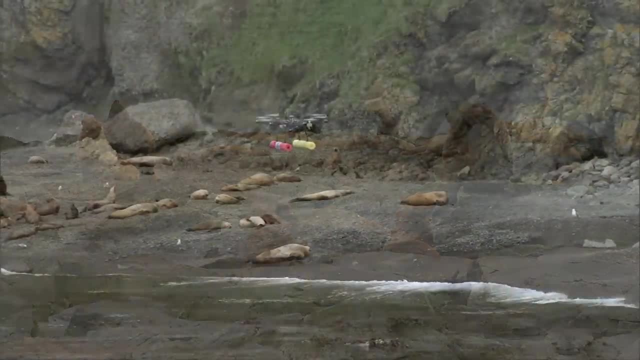 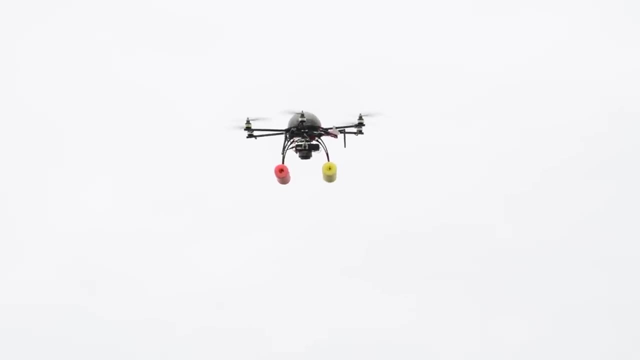 get an accurate count, And it also allows us to do a lot of the work without disturbing the animals. Some of the sites surveyed with the hexacopter in 2014 had not been photographed from the air since 2008.. Together with the remote cameras and continued.